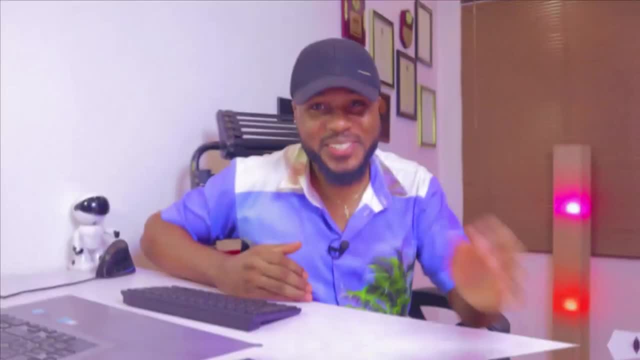 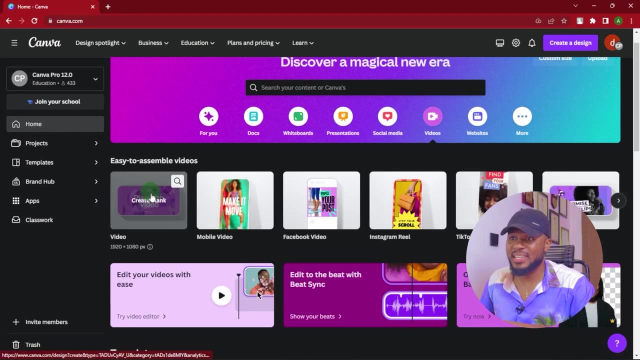 you're interested in, please come closer and let's dive in. So, to get started, fire up your Canva account Now. this is Canva homepage. Come over to videos, click on videos and then click on create blank. So we are going to create a blank canvas and here is the blank canvas. By the way, 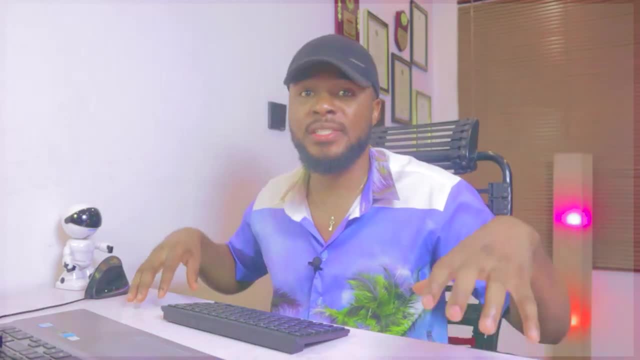 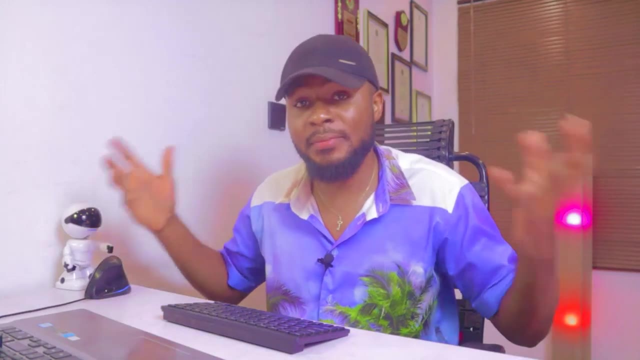 learning how to do this will help you understand how diverse Canva is and how well you can actually get creative with Canva. Now, who would have thought that you can use Canva- the same Canva that we all use- to do our design, that you can use it to do an animation, like a 2D animation? 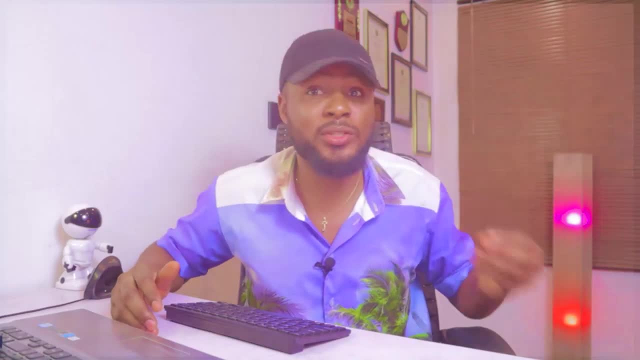 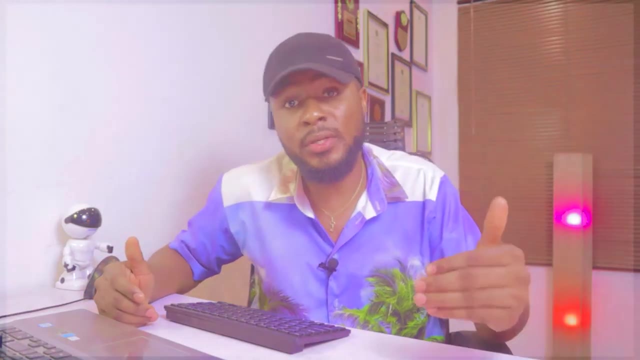 Who would have thought about that? So that is why I want you to learn this, so that you can actually let your creativity run wild, Because I mean, using Canva for things like this means that there is still more out there that you can. 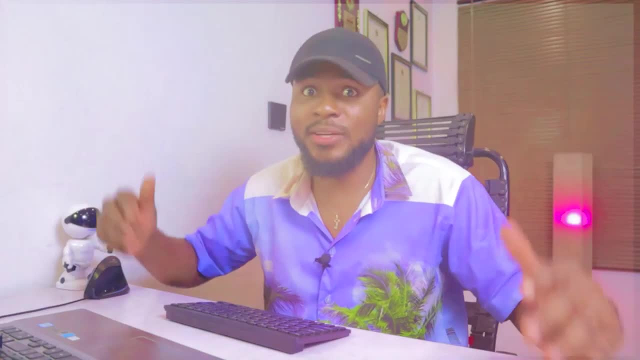 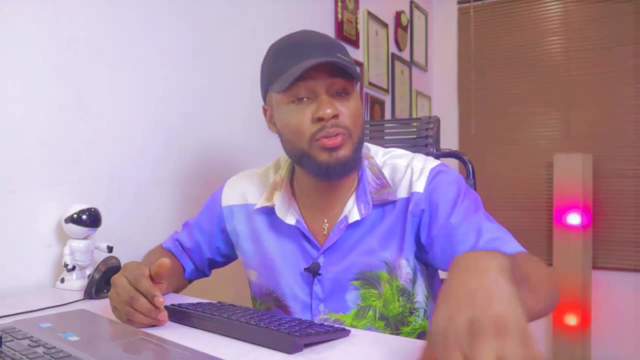 use Canva, for You just need to let your creativity run wild and then you have so many amazing pieces that you can use to wild the world, use to increase your business, use to increase your engagement, use to increase your retention and everything. So, if you learn how to do this, very 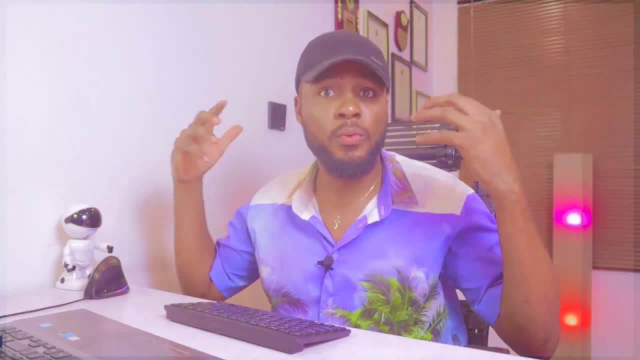 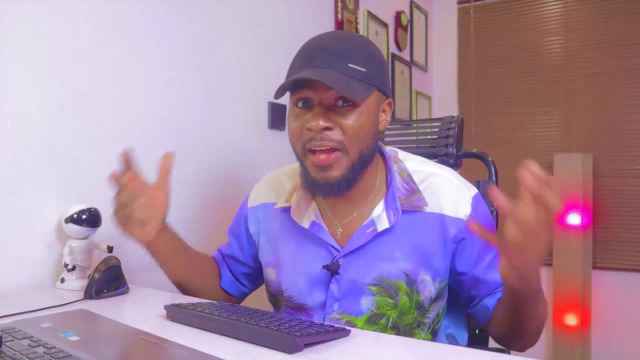 well then, you can actually use it to do anything. You can do the one for cars, the one for houses, and do a voiceover and add to it and actually sell it on marketplaces like Fiverr and all the rest of them. So please, let's continue. 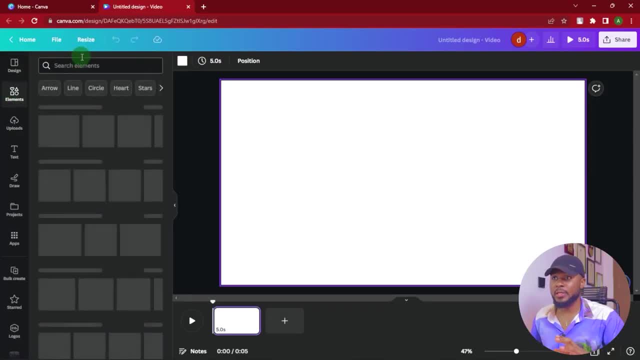 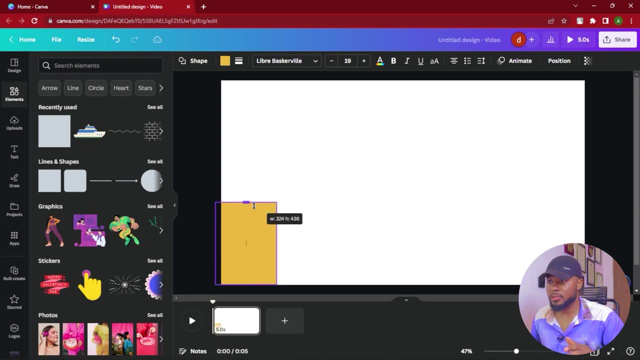 And then the next thing you're going to do is to click on elements. click on elements and click on square, So you select this square and drag it to this place and drag it like so, and drag it like so here, All right, And then duplicate this. You can choose to duplicate this or drag in another. 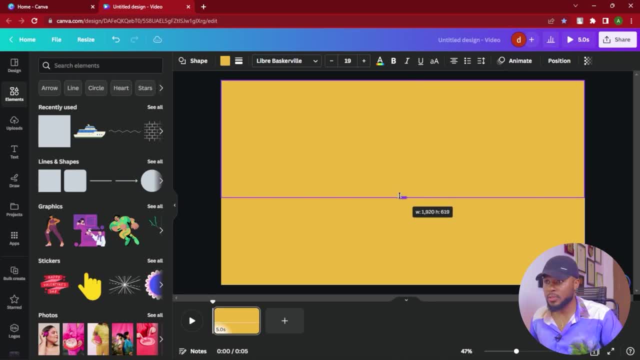 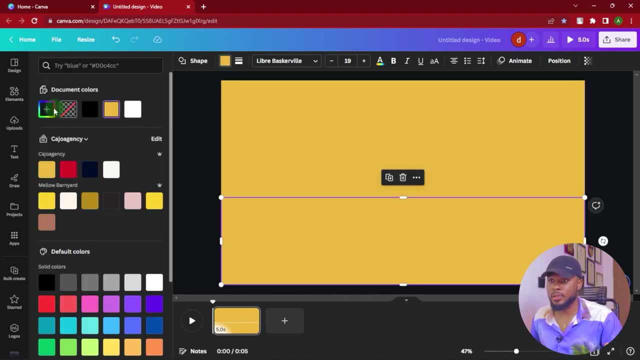 element, It doesn't matter, So, but all you have to do is just create another element. So, but all you have to do is just create another element. So, but all you have to do is just create another element, And you have two elements in one, So here we can change this color to something close. 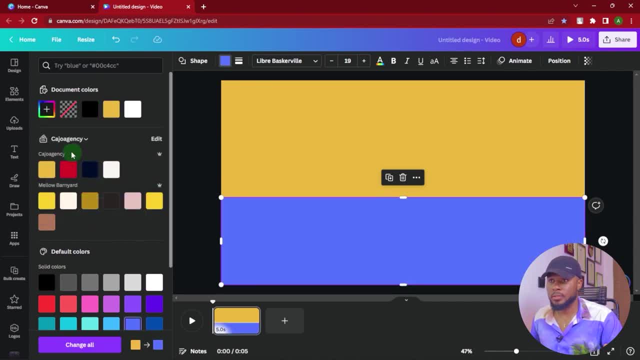 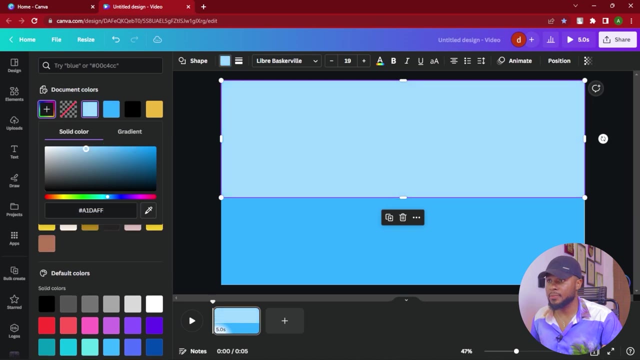 to blue here, So we can change it to this. Yeah, Right, So here you can change it to something like this, A little bit lighter. Yes, So we have this now, And then the next thing you want to do is to: 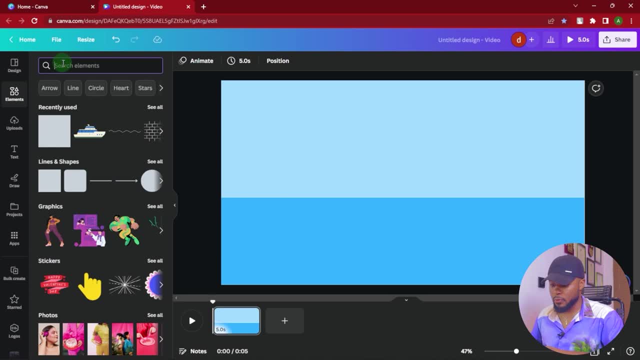 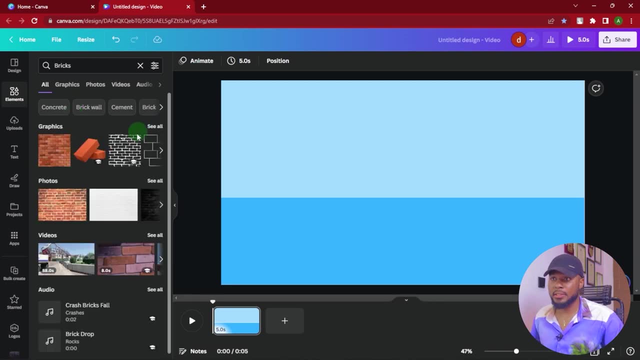 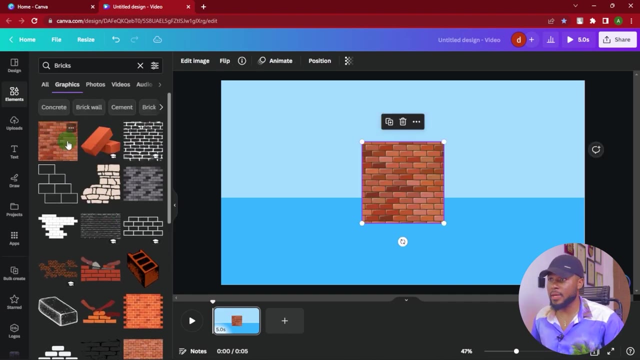 do is to come over the same elements. You come over and search for bricks, All right. So you click on bricks and you select the brick that you want. So we're going to go ahead and click on graphics. So here you select the best brick that you want. So I'm going to go ahead and use this. So all I 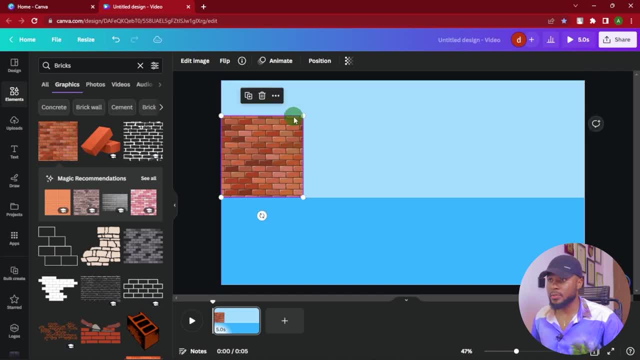 have to do is to come over here and drag it here and resize it to this level to duplicate. If you're using a Mac computer, all you have to do is to hold down command and drag it to this level So you can see it's going to duplicate And then D is going to duplicate. Or if you're using a Windows, 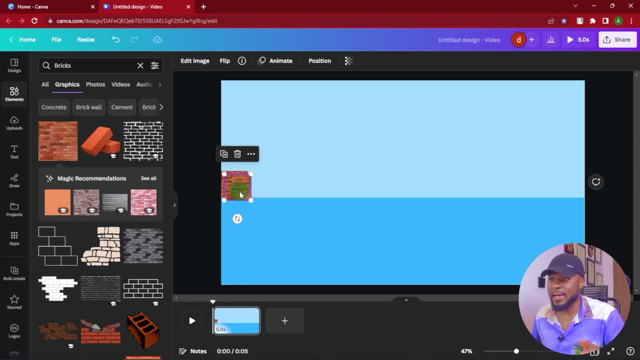 computer. all you have to do is to hold down control and D, and then it's going to go ahead and duplicate. So here we'll have the duplicates and make sure it's well aligned. Then all you have to do is to hold down the control or the command and then keep pressing D till it gets to the end. 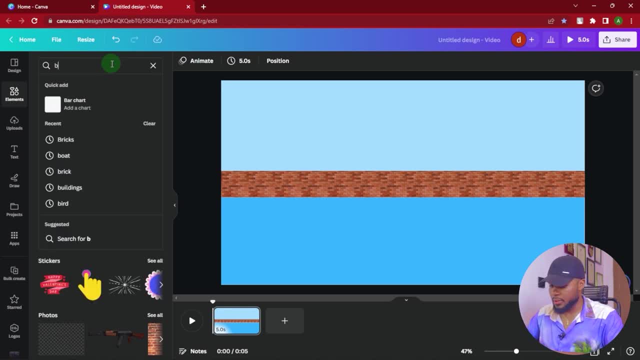 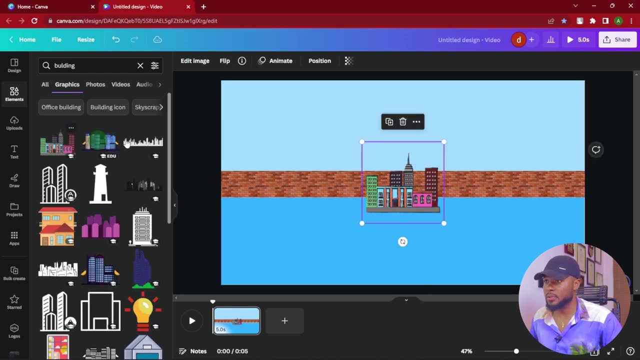 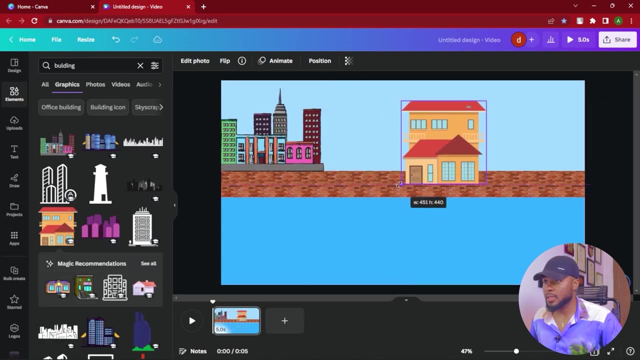 So here we'll have it. And then the next thing we're going to search for is building. So we're going to have building here. So go over to graphics. here We'll have this building here. So let's choose this and then drag it up all the way up, And then we'll have this. Also resize it to fit. 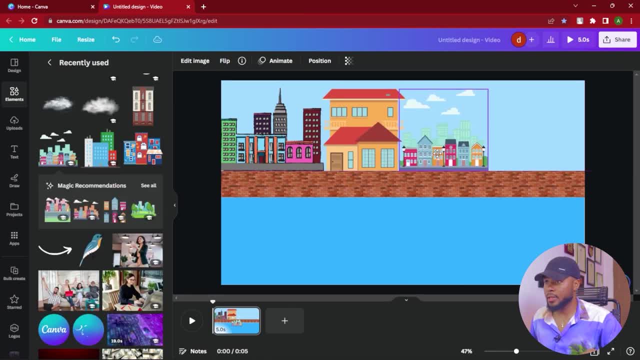 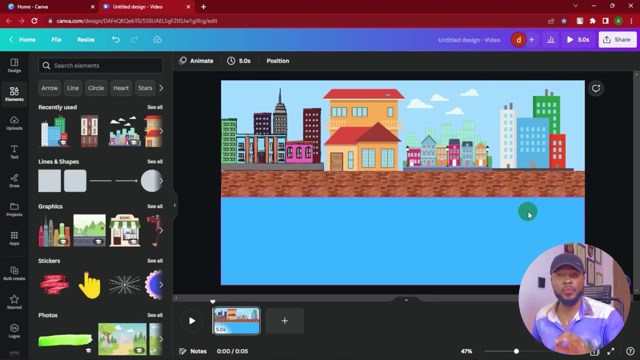 And then we'll select another building and put it right here. And then we'll select just another building and put it right here, And then we'll select another building, like so, and put it right next to this. So now we have the buildings And then the next thing we're going to do is to bring 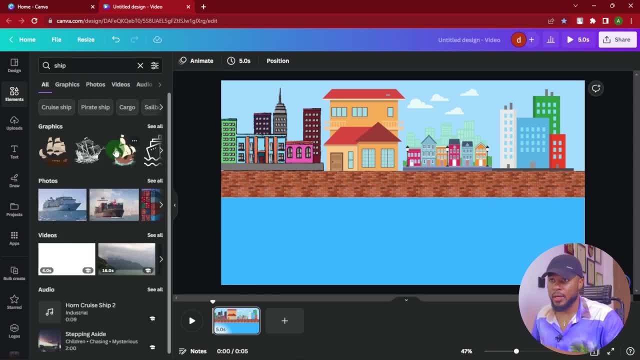 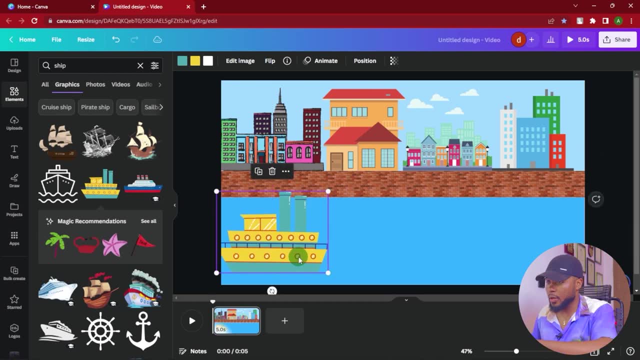 so I'm going to go ahead and search for sheep and click on graphics- Remember, we're using just graphics, So you can use either this or this, Anyone that suits what you're doing. you can choose anyone that you want, But I'm just going to go ahead and go with this And we are almost. 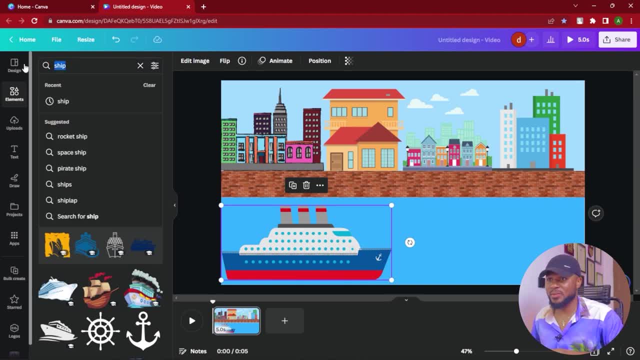 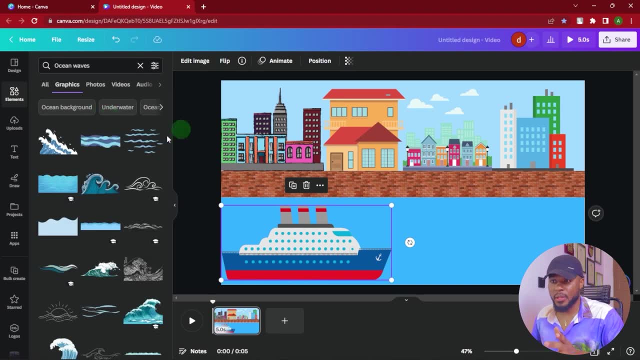 ready. It's just that simple, right. So the next thing we want to do is to add waves, ocean waves. You can add ocean Waves or water waves- anyone. water waves, ocean waves- anyone is fine. So here is a good wave. 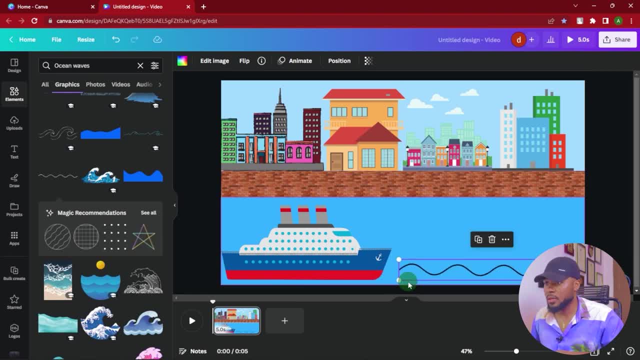 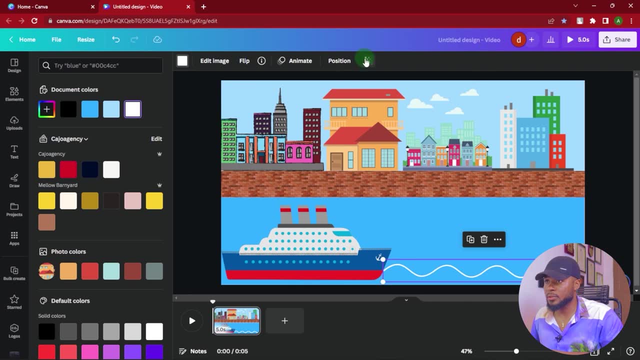 You can choose to use this here. OK, so we can use this as one of the waves and then change the color to white and reduce the opacity to maybe 38.. 38 is fine. And then, and then you duplicate this. duplicate this to: 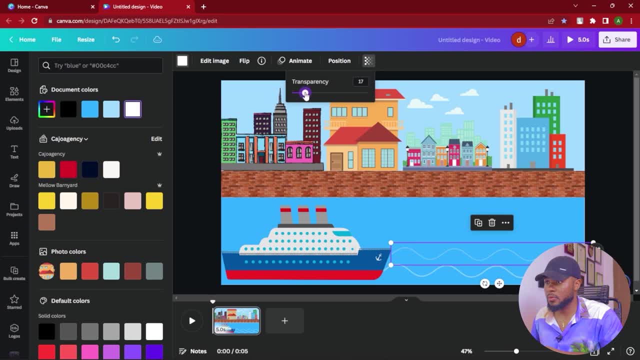 fit in. I think we should just reduce the opacity more. Yes to 12.. So the opacity at 12 is much better. So just do 12.. You just do 12.. The opacity is 12.. So we'll have something great like this: 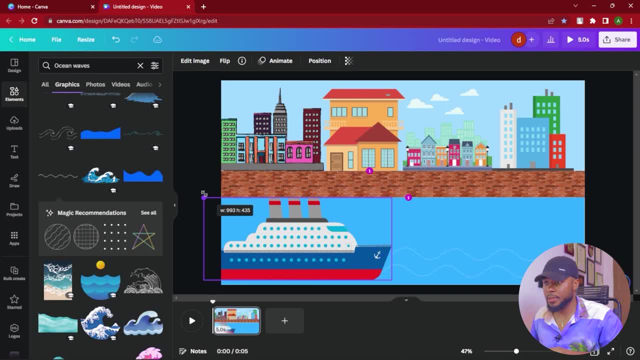 We'll have something like this and then make the sheep a little bit bigger, And we'll have this right. So now everything is ready, but not completely ready. Then the next thing we're going to do is to add clouds. We already have something similar to that here, So we're going to search for clouds. 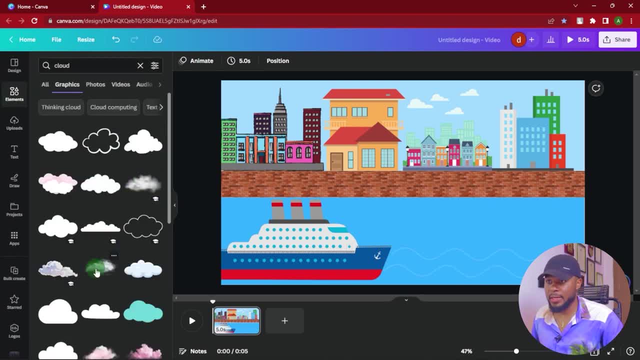 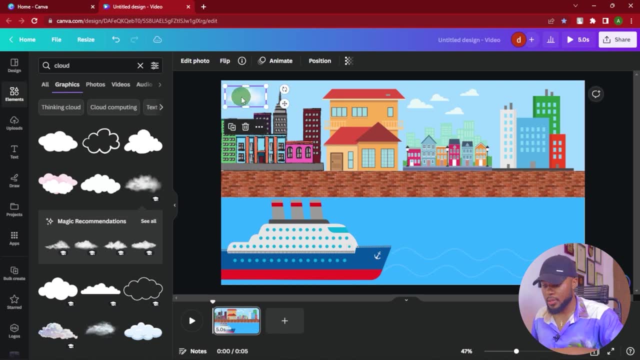 So here is the cloud, So we're going to choose just about anyone like this: Reduce the size and hang it in here, and duplicate this and bring it in here. Now we have our cloud, so we can also do something like this: Put this one here. 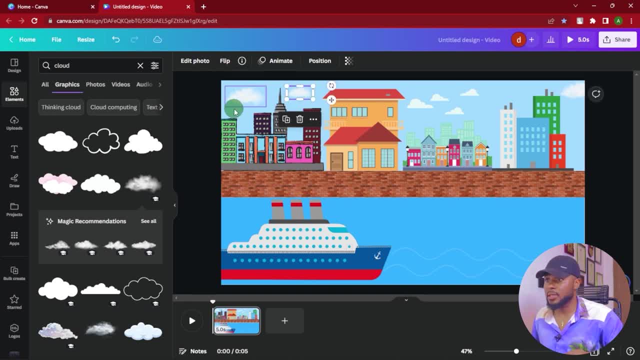 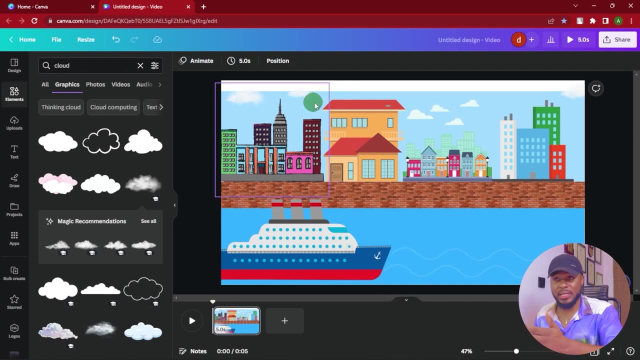 make it a little bit smaller and we'll have something like this. So now we have our cloud, something like this. Again, you can choose to make this whole thing come a little bit down, so there is space here. Now let's go over to layers, because the background has been affected. 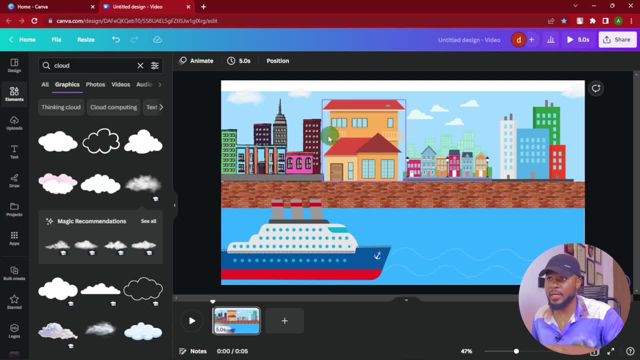 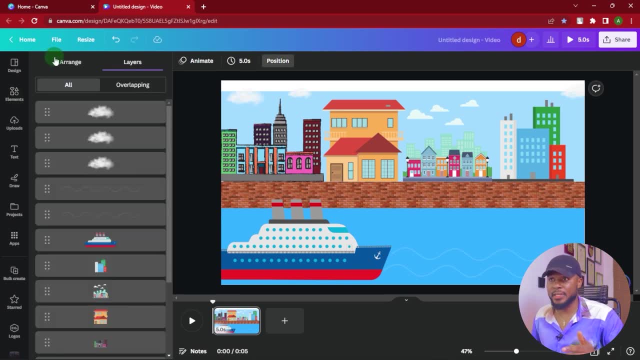 it came down with this thing, so I need to adjust the background and take it up. There's no way I can assess the background now, so the best thing to do is to just click on position and then you have layers here. Now, if you have not seen the tutorial that I made where I showed new Canva, 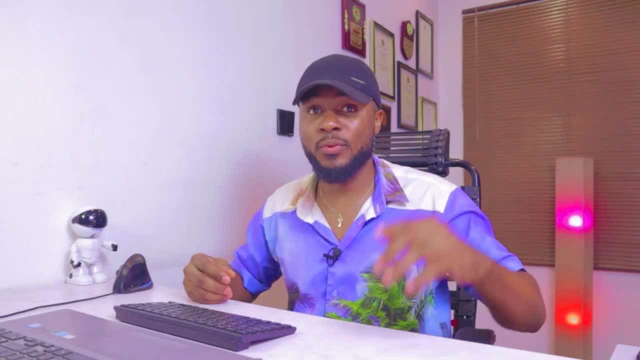 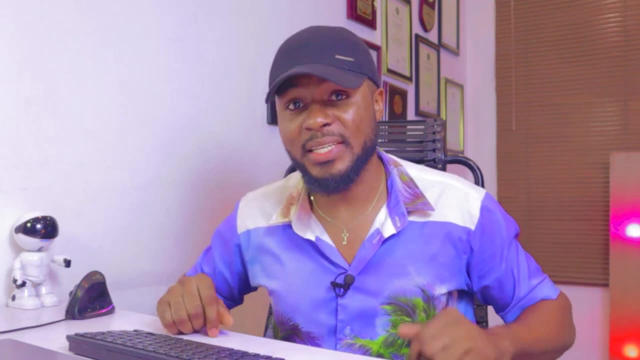 features that you need to know, then please go here right now and watch the video. Click the card here and watch the video, of course, after watching this particular video, and I'll also leave the video link in the description so that you can watch it. after watching this video, of course- and, by the way, 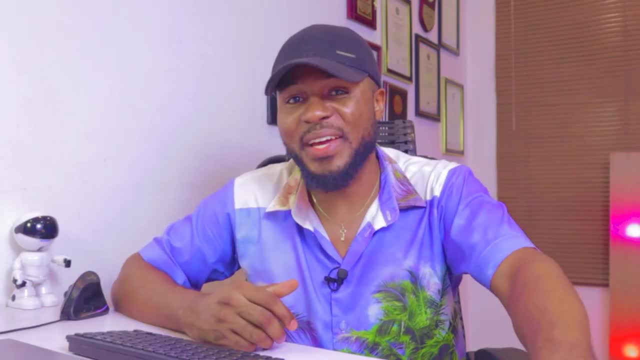 if you have not liked this video right now, I don't know what you're waiting for. please go ahead and smash the like button. It's also a way for you to tell me that I'm doing a good job. so if you think that I'm good at this video, then please go ahead and subscribe to my channel. I'll see you in the 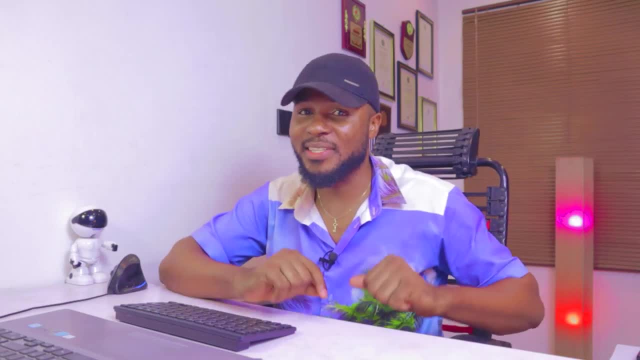 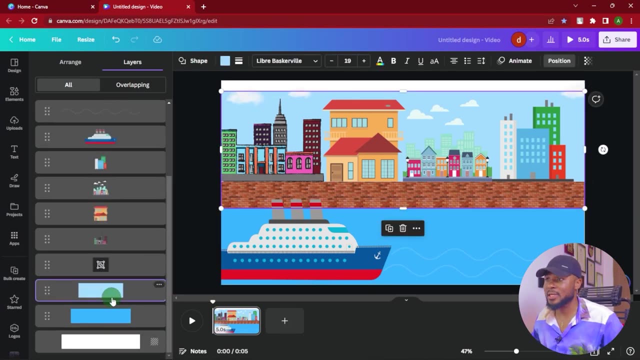 next video. Bye, bye, good job. it's not going to cost you anything. go ahead and smash the like button right now, thank you. so we jump right back and we're going to move the background, which is this: we click on this and you can see it's already highlighted and all I have to do is to just take it up. take it up to. 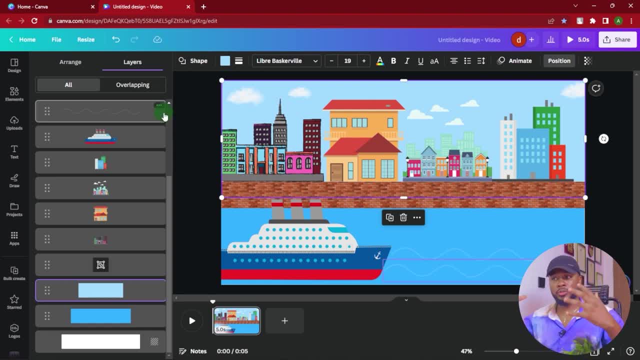 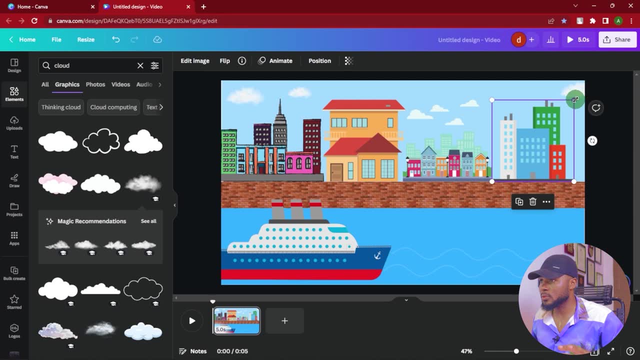 this point. so now we have something like this: it's no longer, you know, choked up. so, um, we'll have our design ready and good to go, so I can decide to raise this one up a little bit, to be a little bit taller. yes, to be a little bit taller is is better. so this is good, like this and raise this one a. 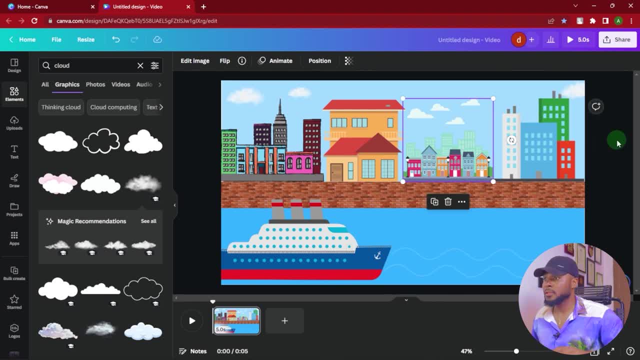 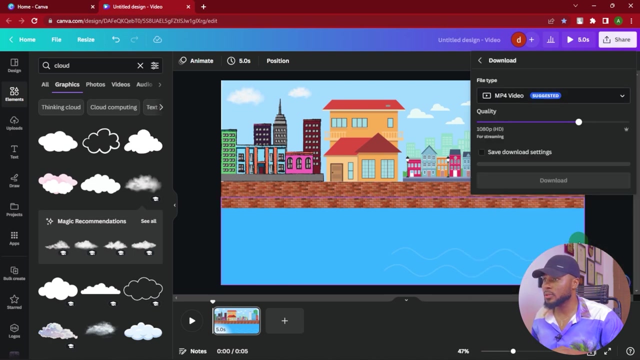 little bit. yeah, so we have something good, so this is an amazing one we have right here. so the next thing we want to do is to take this whole project to CapCut and animate it, and the process of this is to cut out this here and go over to share and come over to download and then come over to 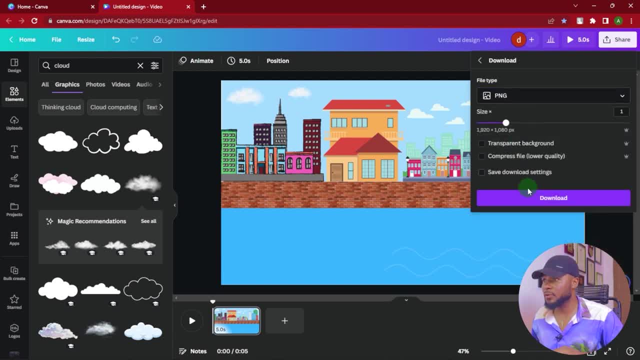 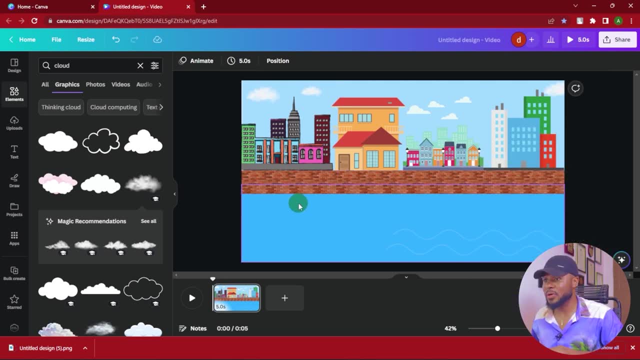 file type and click on png, select png, of course, and then click on download and we'll have it downloaded to our device. now it's downloaded to our device, and then the next thing we're going to do is to create another fresh page and paste the sheep that we copied. we're going to create 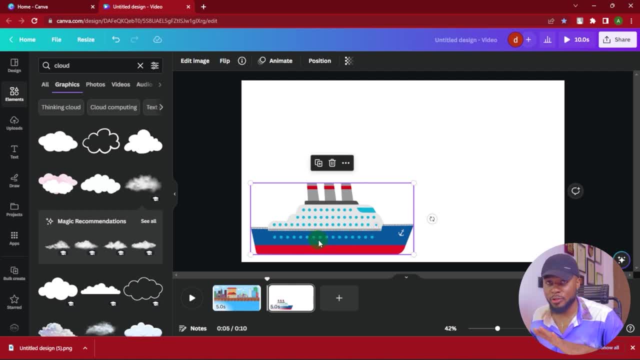 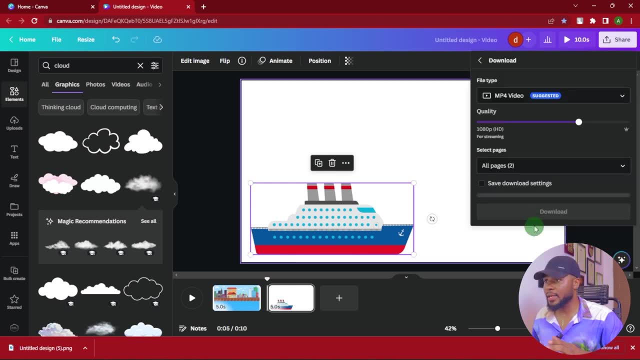 to paste it like this: the same size. please do not do not resize it, just paste it as it is and then click on share again, and click on download again and come over here and select png. and now this is where it gets interesting. this is something you must do. click on transparent background- okay. 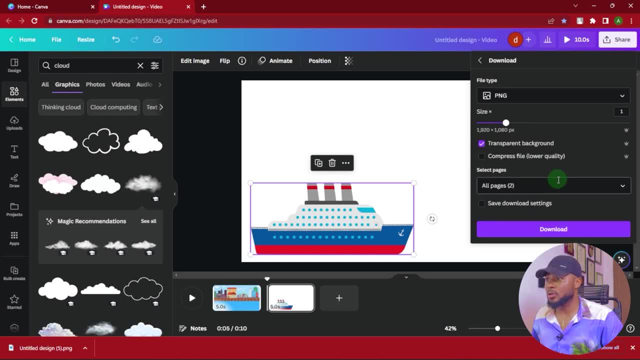 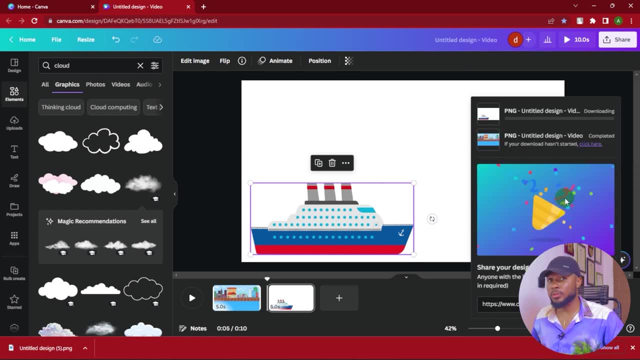 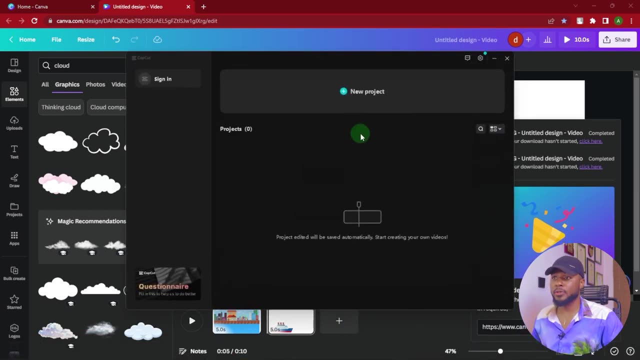 make sure you select the transparent background. and then you come over here and select only page two and click on done, click on download and it's going to download straight to your device and that is it. and then we'll jump over to CapCut here. so this is our CapCut. you can access it with. 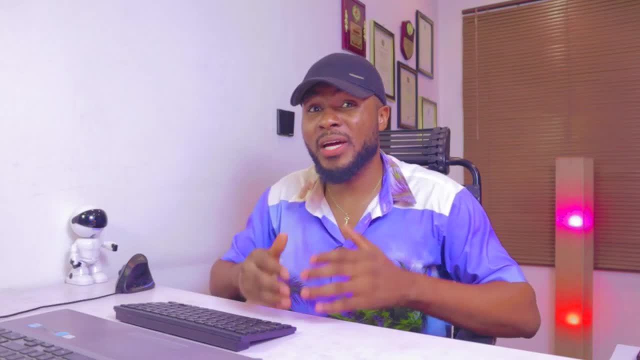 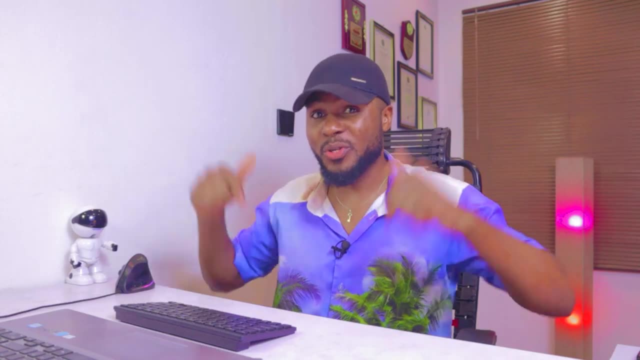 your phone or with your computer. i've done a CapCut tutorial where i broke down CapCut walkthrough. please click this card here now to watch the video. of course, after watching this video, but i'll also leave the link in the description as well, so that you can watch. 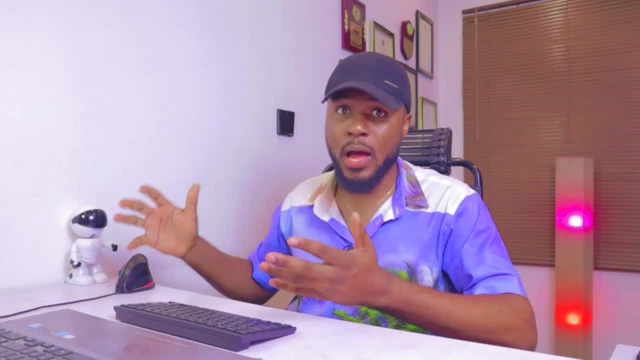 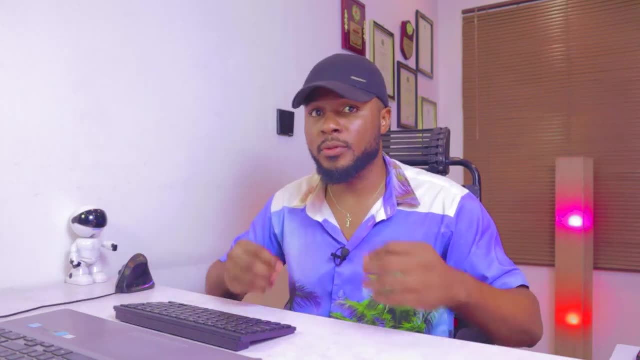 the video after watching this one, so you can best understand how CapCut works. just in case you're new to CapCut for desktop or you're new to CapCut entirely, but you can do this with your phone as well as do it on your desktop. so here you click on new. 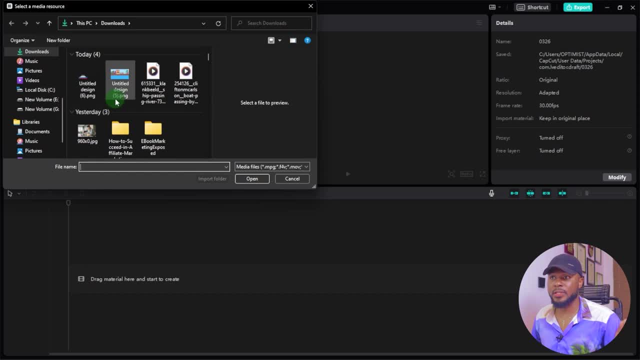 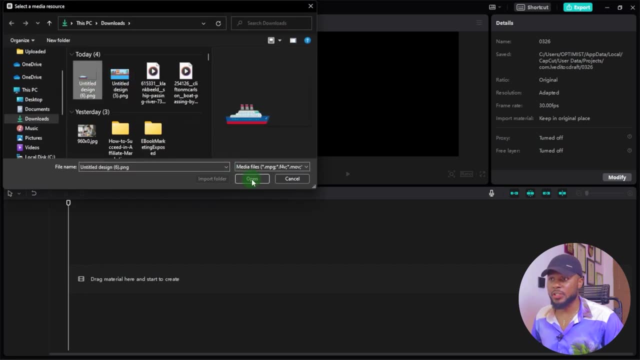 projects and then click on import. so we're going to import the picture that we downloaded, the first picture, we're going to import this one and we're going to go ahead and click on import again and import the ship, and then we'll have the two and then we'll drag this to the timeline we can make. 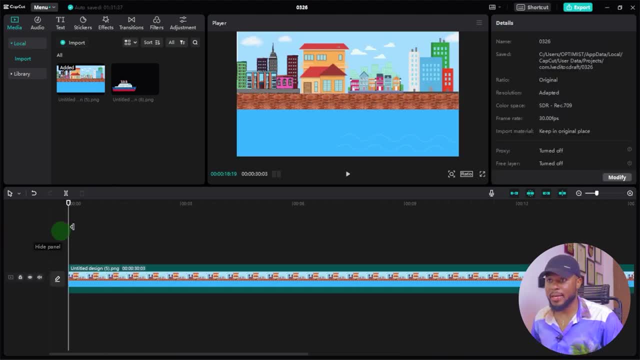 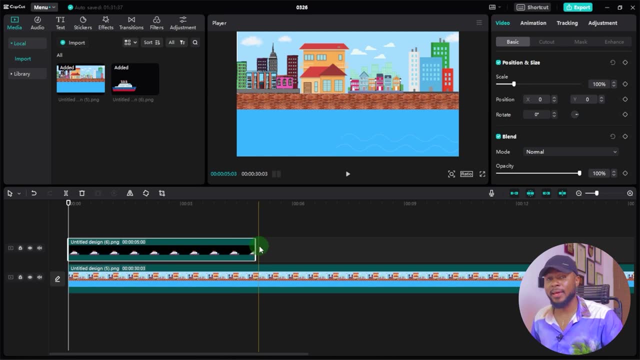 this longer and we'll come right back and see how CapCut works. just in case you're new to CapCut, select the ship, drag it on top. if you're using the mobile phone, all you have to do is just click on overlay and bring in this picture. so just click on overlay and bring this picture. if you're using 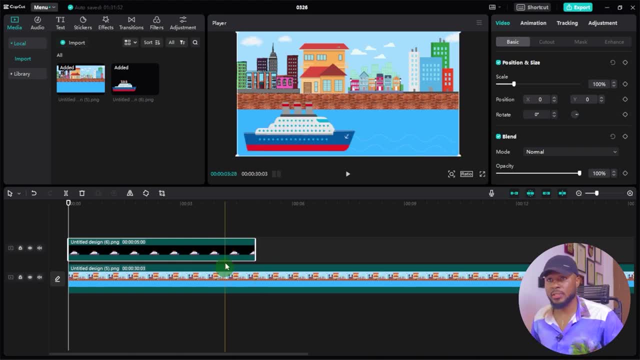 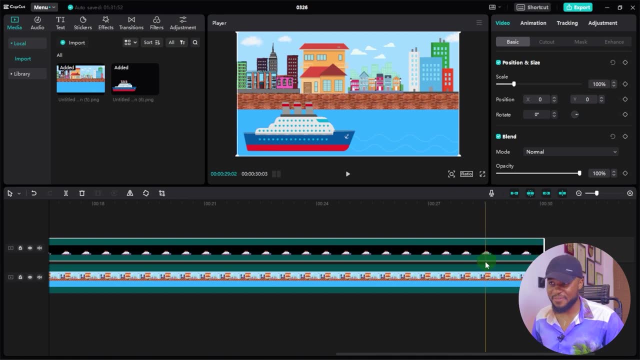 it on your mobile phone. so it's just the same thing. this is just an overlay, right? so you work with overlay. so now we have the exact same picture that we have on Canva. now, this is where it gets interesting. this is where it gets interesting, guys. please pay attention. so here, all you have to do is 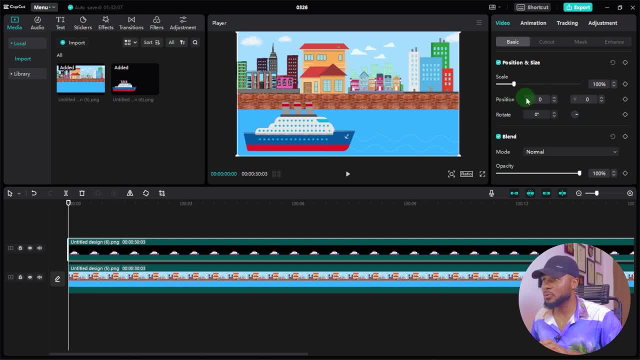 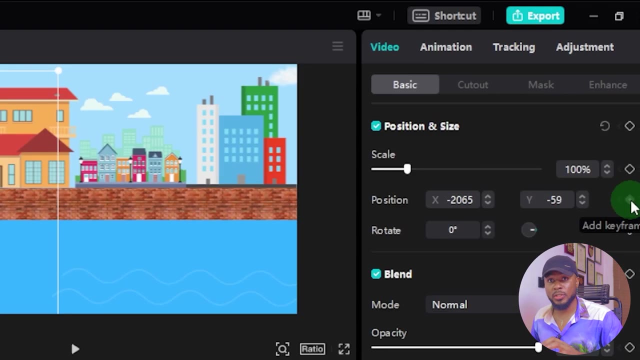 click on this ship right now and you have this position and size. so this position and size, all you have to do is to click the picture and then take it way back. take it way back just out of the frame and then. so you just click here to add a keyframe. so you click here to add a keyframe. 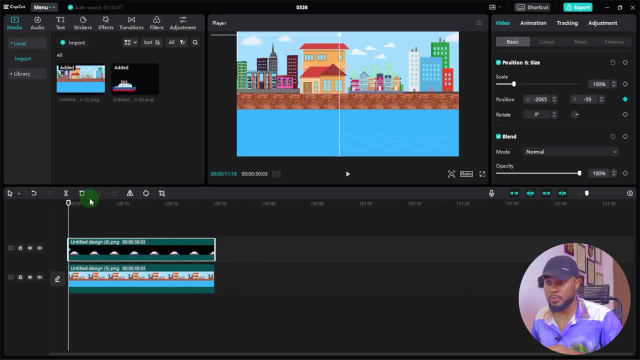 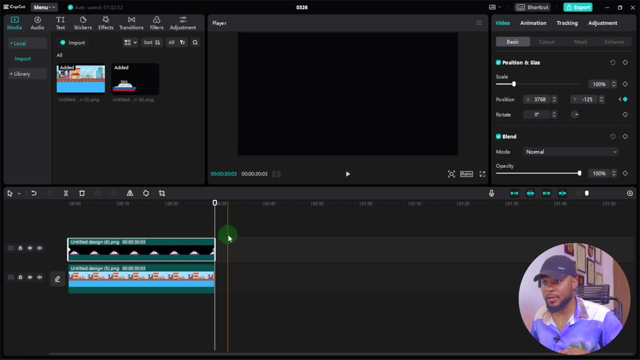 and then you bring this one back to this point. so you bring this one to the end and bring back the picture to this point. bring back this picture to this point where it's off the frame again and you have another frame automatically. so if I scrub through, you can. 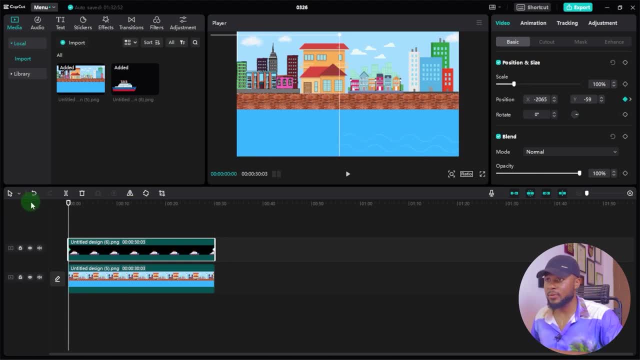 see that it's now working. so if I play it right now, you can see how it is. so the next thing I want to do, let me increase this. so the next thing I want to do is to make sure that everything is the way it's actually coming from up, and then it went a little bit down, which is very perfect. 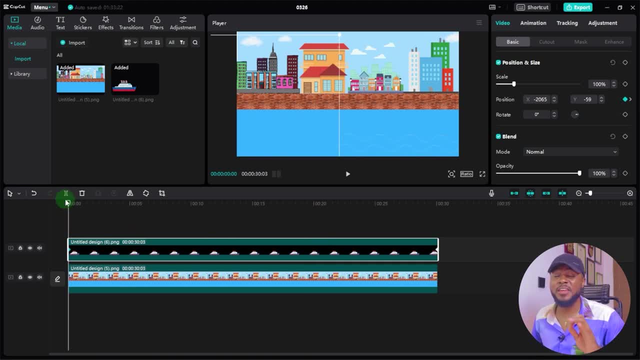 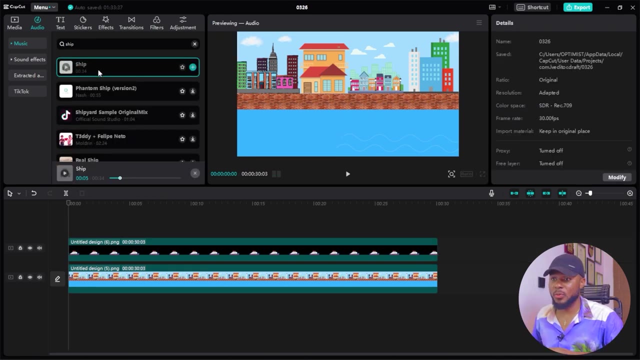 now the next thing you want to do is to add sound, to make it even more realistic. now to add the sound, all you have to do is to come over to audio and search for sheep. simple, simple, okay, let's ask for sheep. so here we have the sheep sound and all we have to do is to drag it to this place and 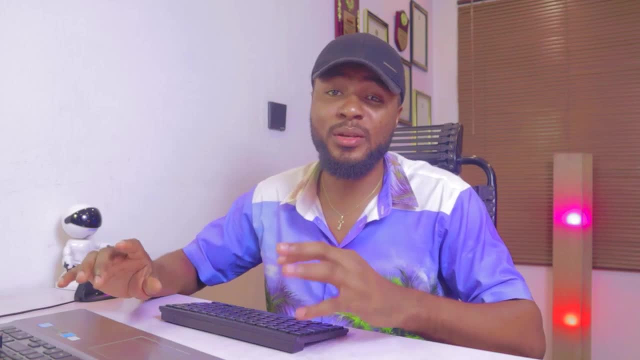 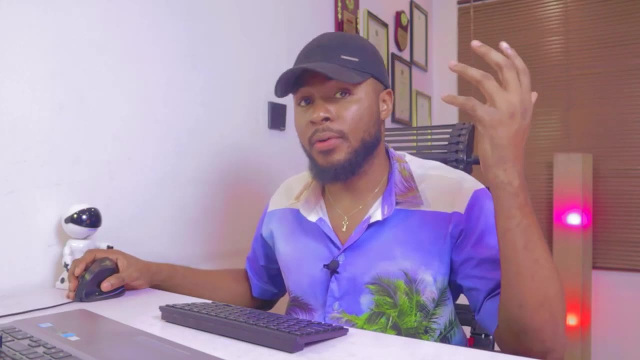 we're going to go ahead and resize it to this point. we're going to download bird, flying butterfly and man working. so these are the three elements that we're going to be adding to our, our design. so, now that we have downloaded all that we need to work with, let's now come over to CapCut and 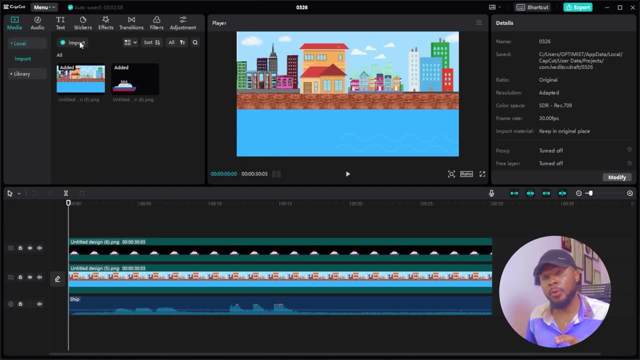 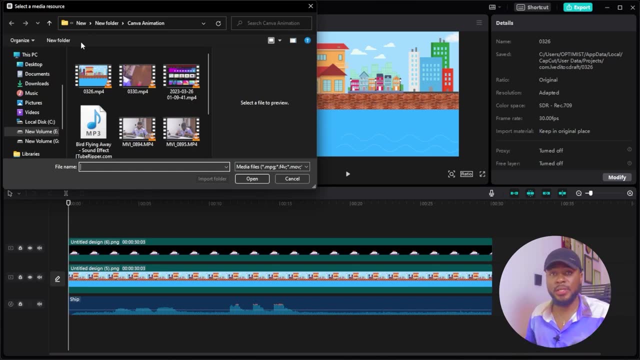 import those things that we downloaded. all we have to do is to come over here and click on import, so that we can then go to where the file is on our system or in our phone and bring in those videos that I just downloaded. so I'm going to show you how to do that now, and now we're going to go ahead. 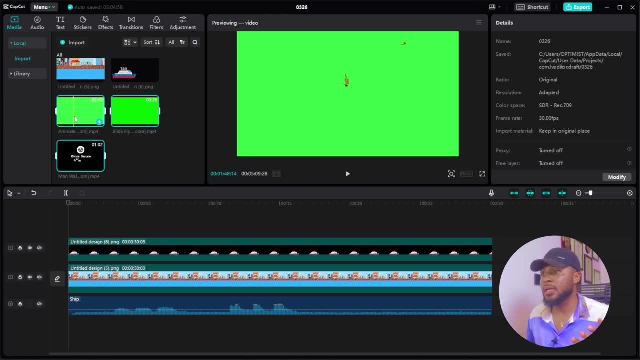 and import those things that we downloaded. all we have to do is to come over here and click on import those things that we downloaded. all we have to do is to come over here and bring in those videos. this is for the animated butterfly, and this is for the birds and this is for the man working. so let's 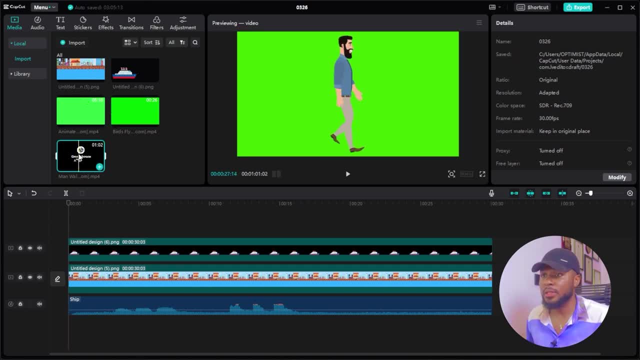 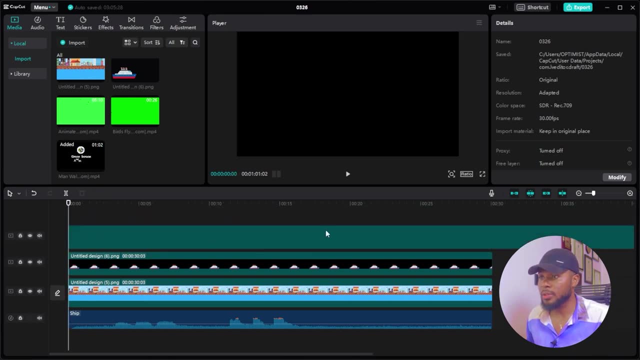 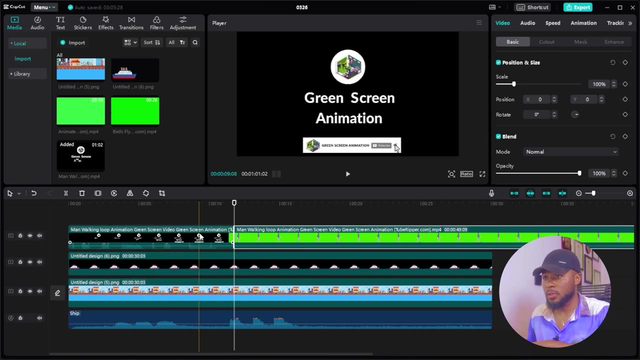 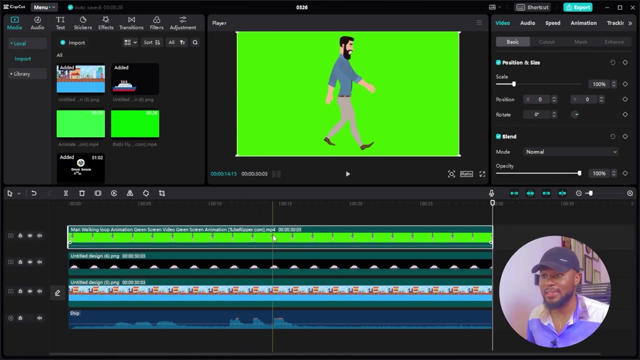 put this now. so first we'll start with the man working and we'll select this video and drop it here. so we're going to cut this off right here, so it will fit into our time frame, so I'm going to and then put it here. so all we have to do is to just highlight the video and then we'll come. 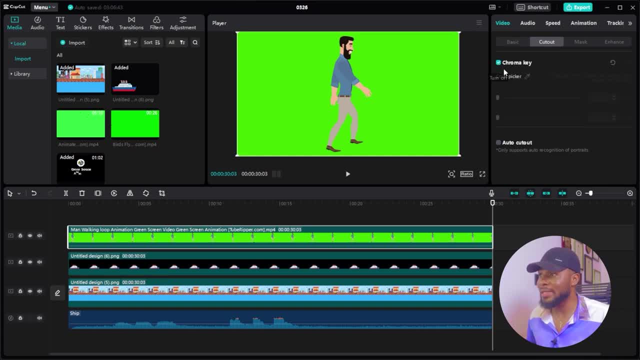 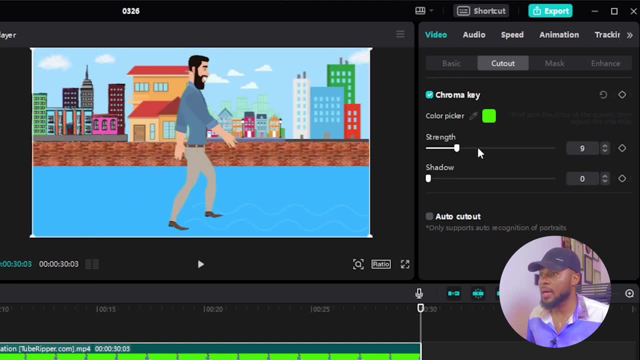 over here and click on cut out, and click on chroma key, and then you click on this color picker and then select the color and add strength, add shadow, or you can remove shadow. I usually leave it like this. so the strength is okay, this one is okay, and then the next thing you want to. 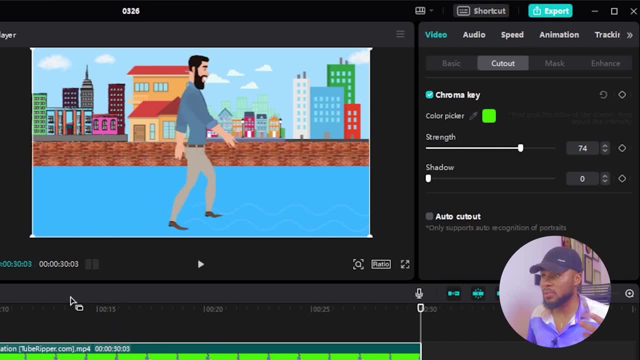 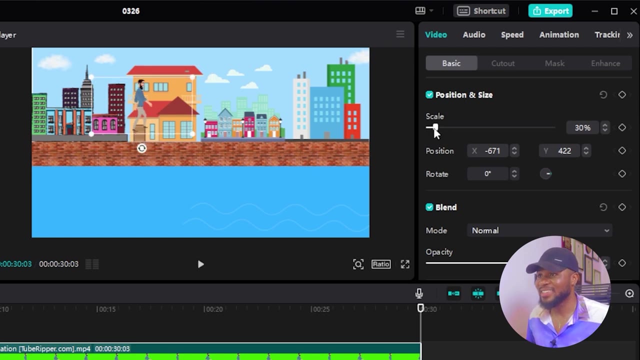 do is to resize. this is to resize the whole thing. so you go to basic and then you go to scale, to resize here, like this, and then you place it here just like this. well, he's like a giant, so we just resize it and put this one here. yes, so let's scale it a little bit more. 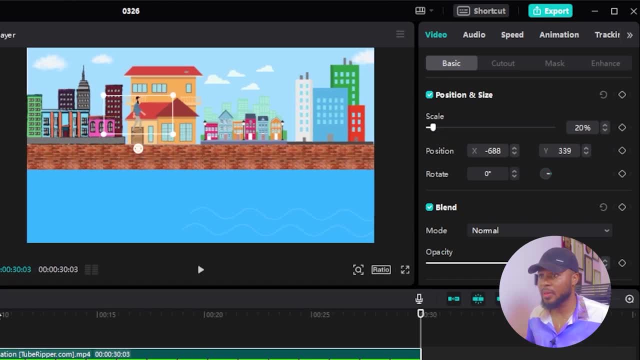 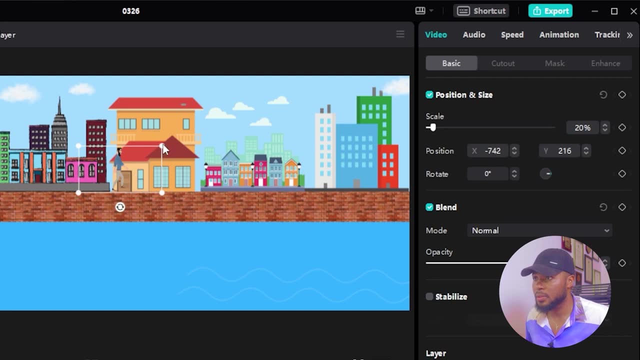 let me increase this one so that you guys can see it perfectly, right? so let me drop this. increase it a little bit more so now you can see if I play it, he's still standing in one place. so for him to move, I'm going to do the same thing that I did to the sheet by using 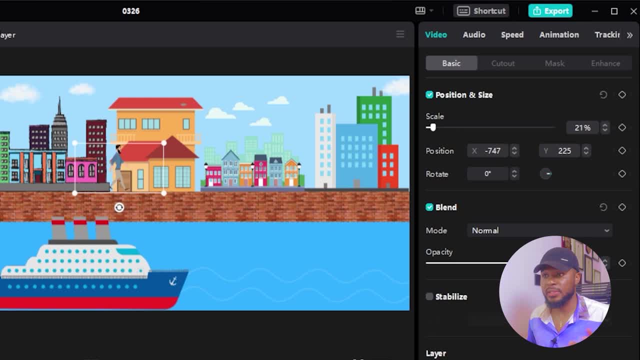 keyframes. so all I have to do is to take this one back, make sure the video is still highlighted and then you come over to position. so the position, you have to add a keyframe. you're going to move it to this place. so moving to this end, because I don't want him to be working too. 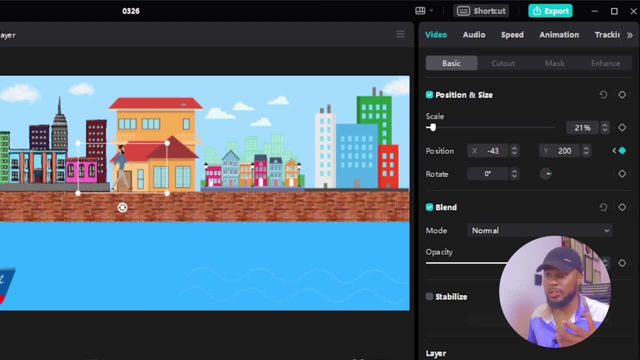 fast, it automatically adds another keyframe, like we did with the sheep. now you can see that he's working a little bit faster. so that is that for demand. so we're going to bring in the beds as well. we're going to do the same thing for the birds: bring in the beds. like so. here is the bed. 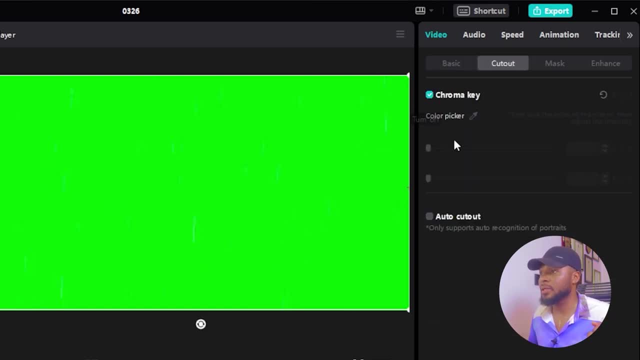 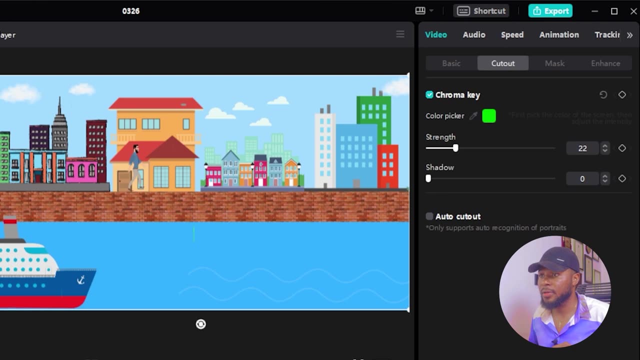 you do the same thing. you go over to cut out and you go to chroma key and then you pick colour pick and remove the background by increasing the strength and then you have the birds flying. so, as you can see, the birds are actually flying in the wrong place, right? so here the birds are. 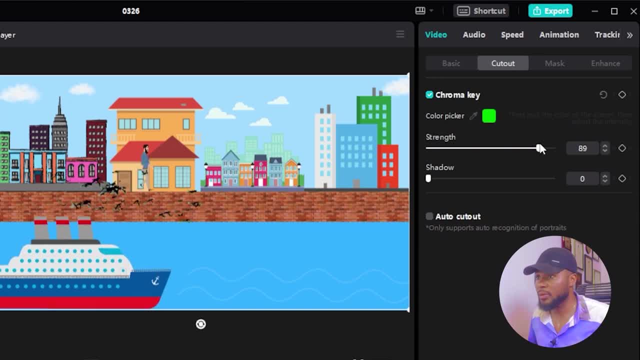 flying in the wrong place and they still have this green screen thing. so we're going to do like so: increase the strength, then increase the shadow, like this. so now we have the birds flying, increase this a little more, a little more. yep, like this, increase a little more and we're good to go. so if 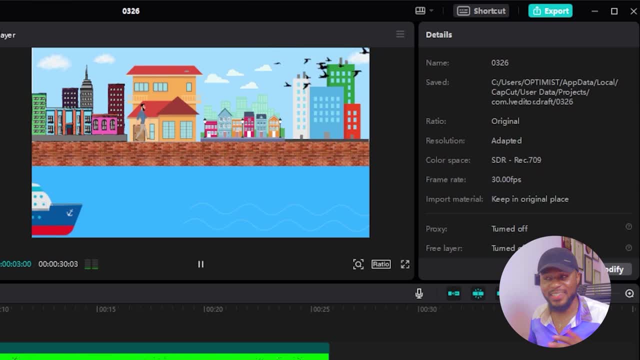 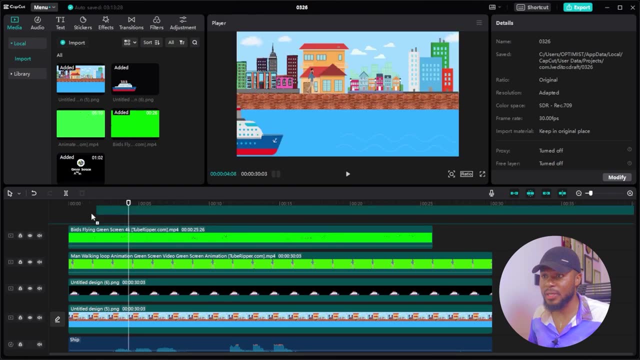 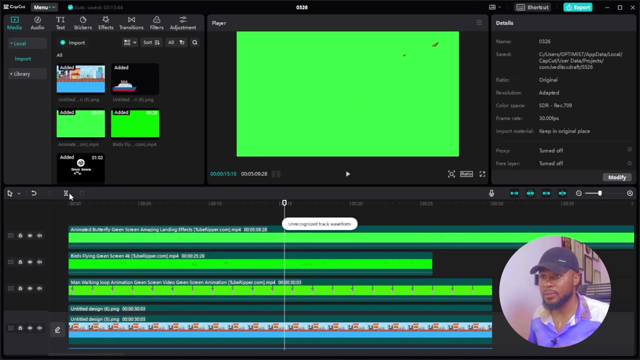 we go back, you can see the birds flying over. all right, so, and the next one is to add the butterfly, add the butterfly effect. so come here, drag the butterfly to this point and choose the point that we want and cut out the rest i'll go to. 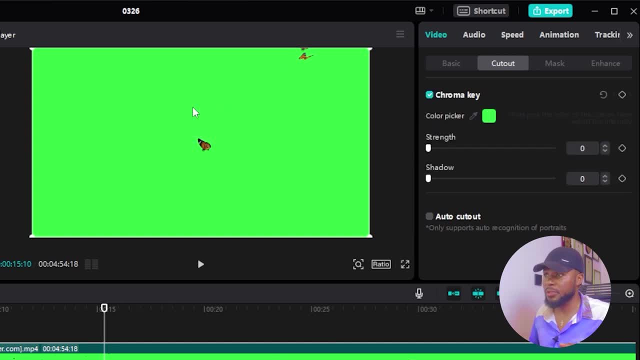 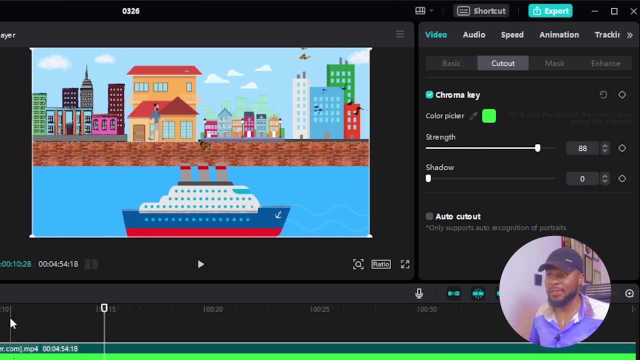 out and chroma key color picker. remove the green screen by increasing the strength and increasing a little bit shadow and we have the butterfly flying. so how cool can this be right? so this is how i've been able to make this animation. to export it: all you have to do is to click on export.